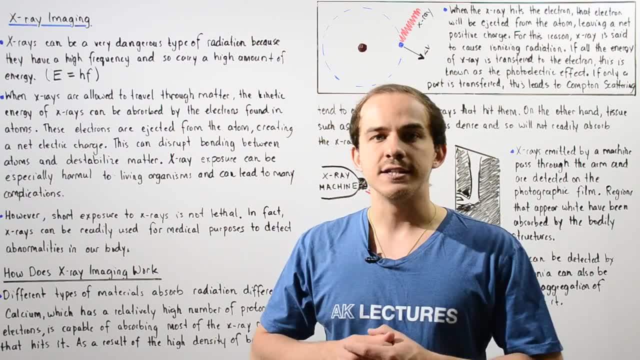 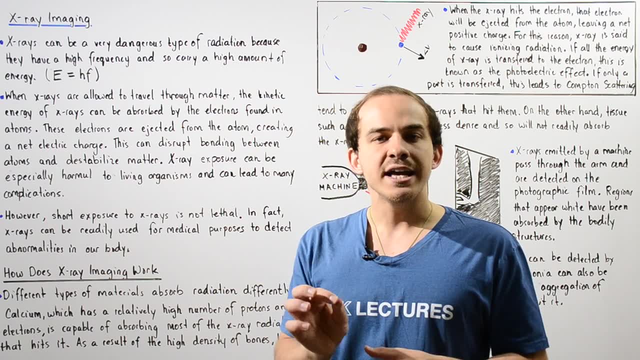 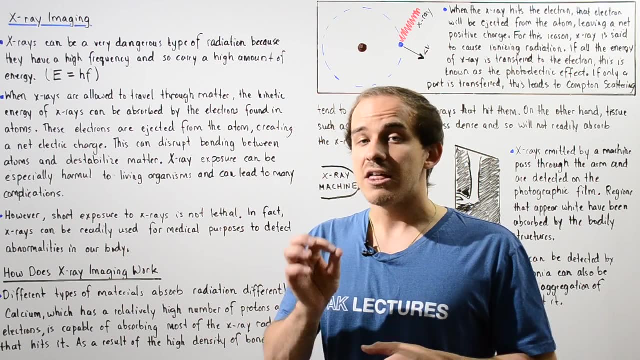 x-rays can be transferred to the electrons found orbiting our atoms And when those electrons gain that energy, they can be readily ejected from those atoms, creating a net electric charge on that atom And those electrons fly away in all different directions. Now, as a result of that net, 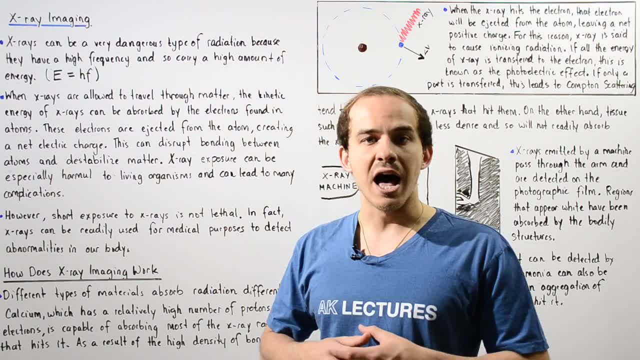 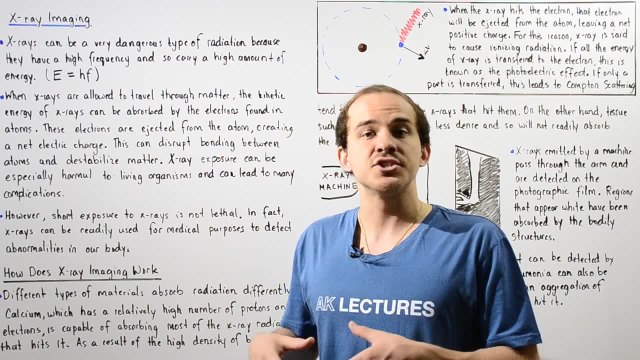 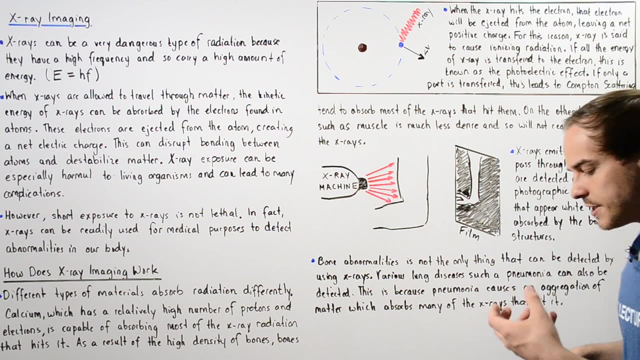 electric charge. this can destabilize the chemical bonds That exists between that atom and some other adjacent atom, and this thereby destabilizes the entire structure as a whole. Now, as a result of this idea, we see that long exposure of x-rays to living organisms can be especially harmful and can lead to many complications. 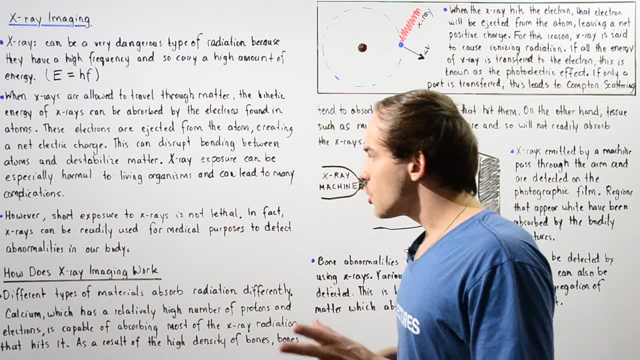 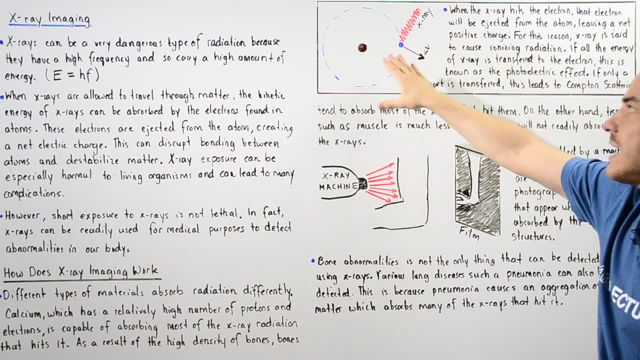 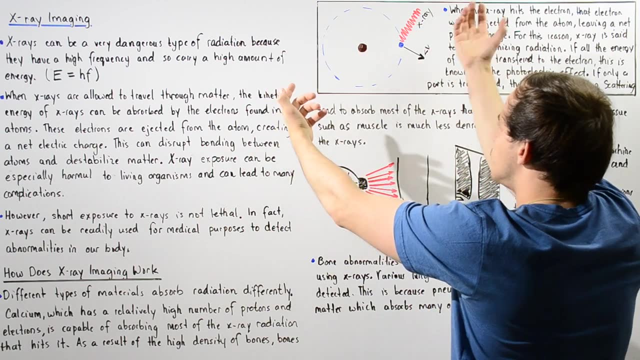 for example, cancer or cell death. So let's take a look at the following diagram, which basically describes how x-rays interact with the electrons of our atom. So we have the Bohr model of the atom, We have our nucleus, the protons and 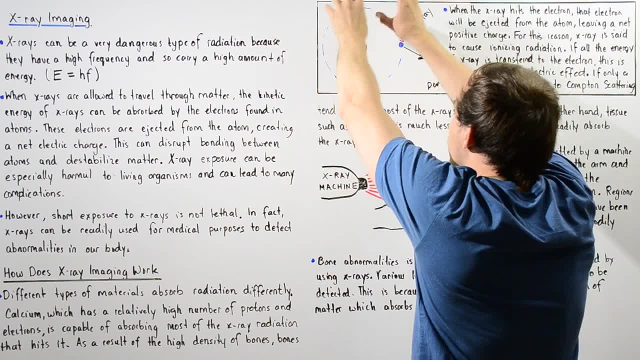 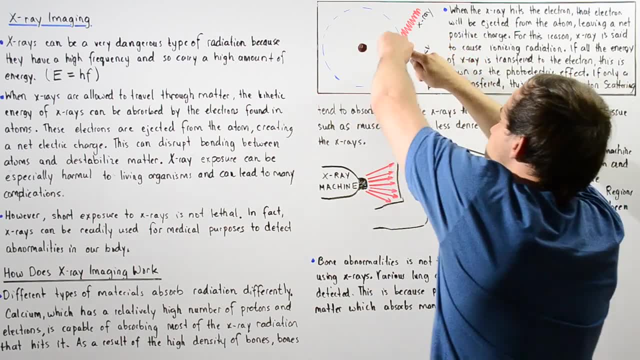 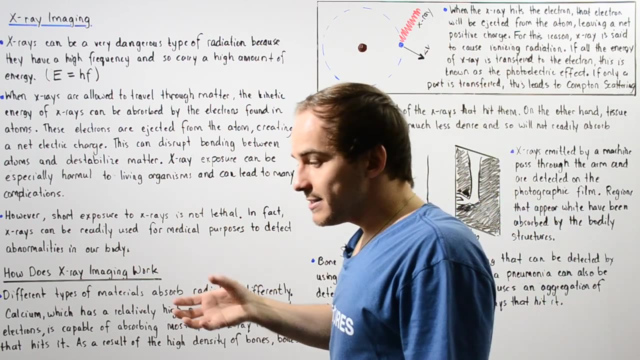 neutrons are found in the nucleus and the electrons are orbiting our nucleus, So they are found within an electron cloud. This is one type of electron. let's say it orbits around the following circular pathway. Now when our x-ray basically hits that electron, one of two things can happen. That electron can 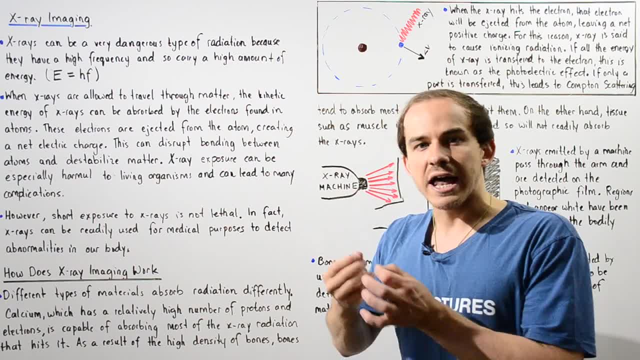 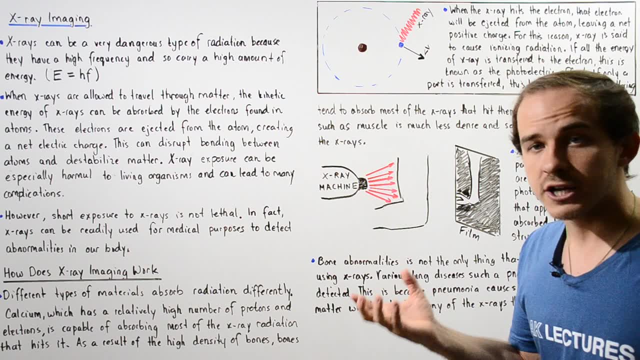 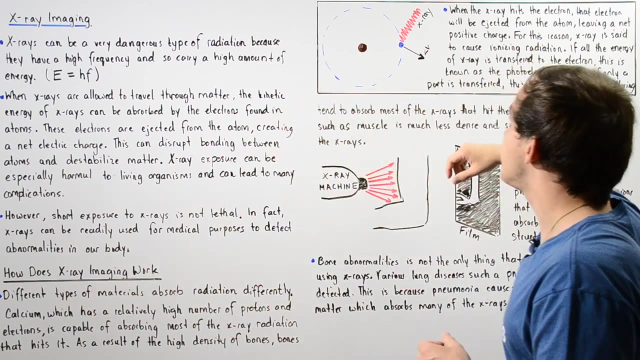 either absorb all of that energy that is found within the photon of x-ray, in which case this is called the photoelectric effect, and the electron gains a great deal of kinetic energy, flying away, ejecting itself, and our x-ray ceases to exist and the entire atom has a net positive 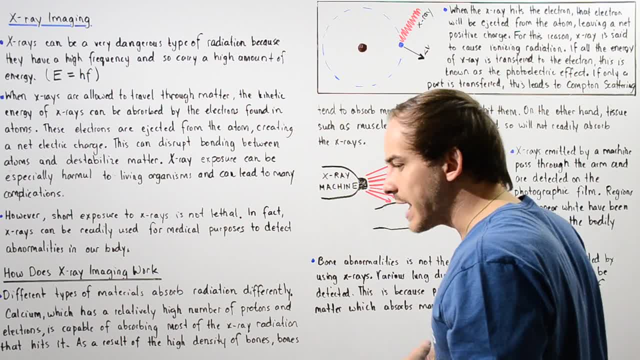 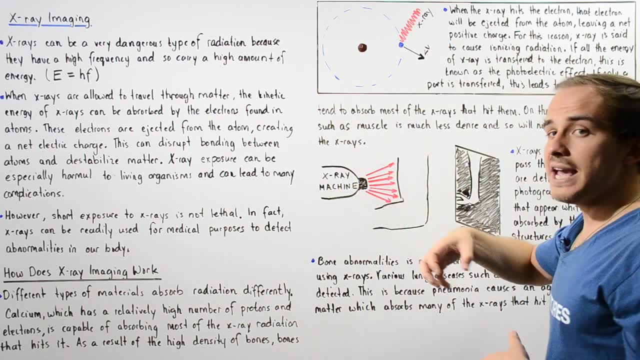 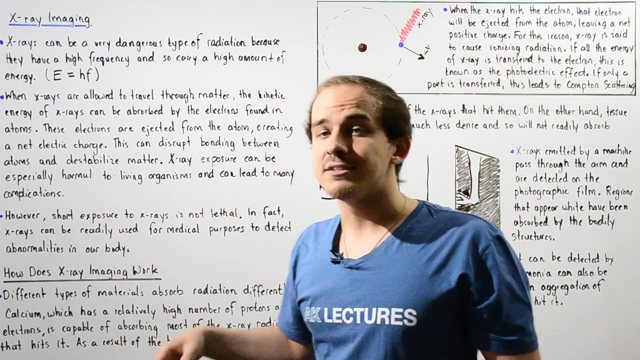 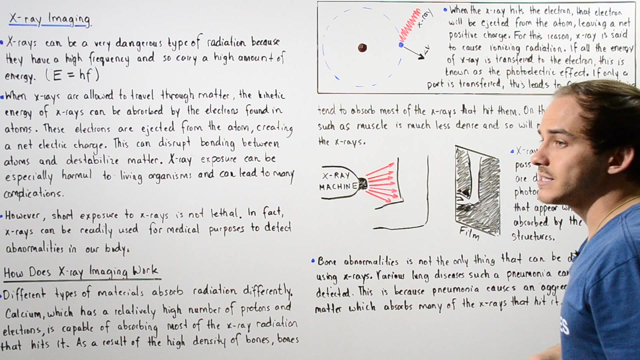 electric charge. Now another thing that can happen is known as the Compton effect or Compton scattering. In this case, only a part of the energy carried by the x-ray is absorbed by that electron. The electron still ejects itself, the atom still gains, or the atom still- yeah, the atom still gains- a net positive charge. 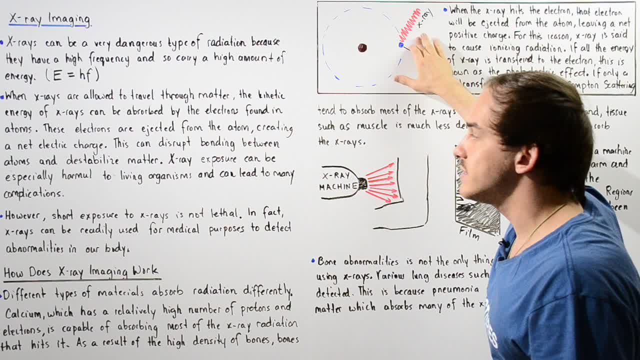 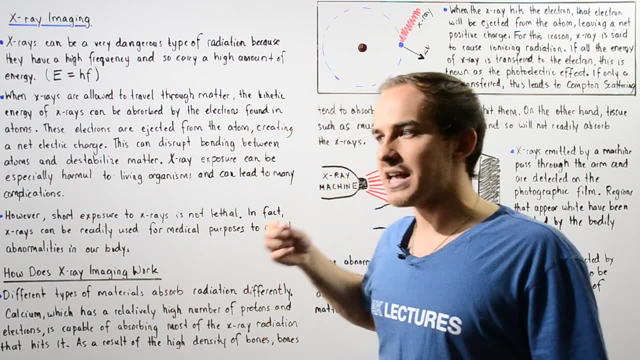 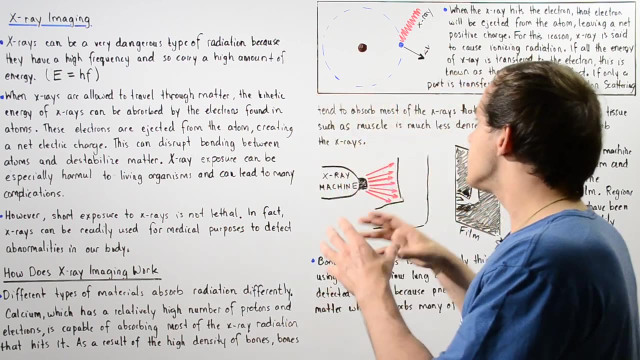 but now the x-ray doesn't cease to exist. the x-ray bounces off and travels outward in some general direction, and this x-ray can then hit another electron found in another atom, further destabilizing the entire structure. So, once again, when the x-ray hits the 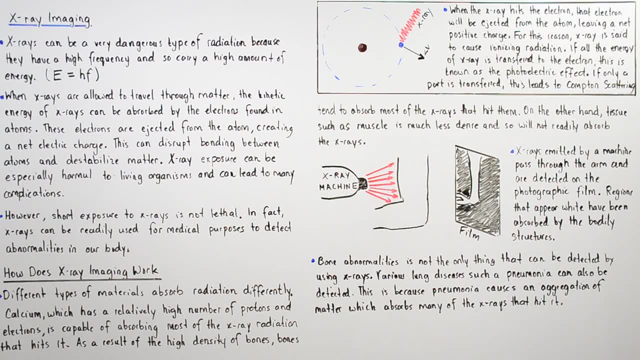 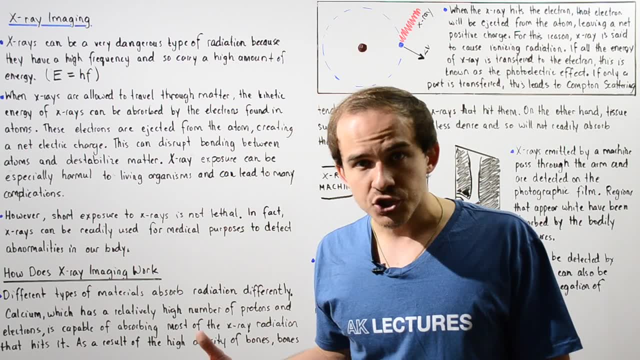 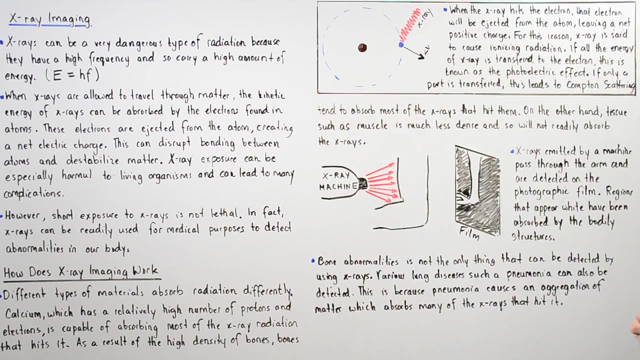 electron. that electron will be ejected from the atom, leaving a net positive charge. For this reason we call x-ray radiation ionizing radiation, because x-rays ionize atoms. they create charge. So if all the energy of the x-ray is transferred to the electron, this is known as the 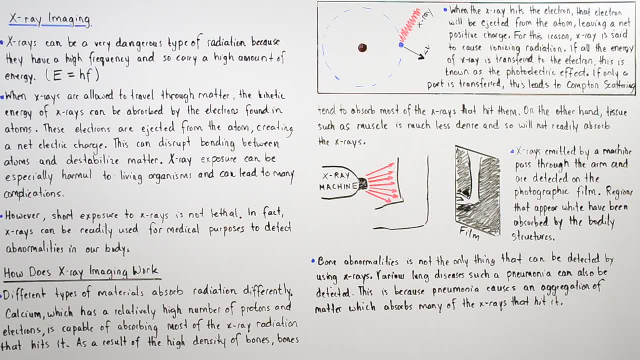 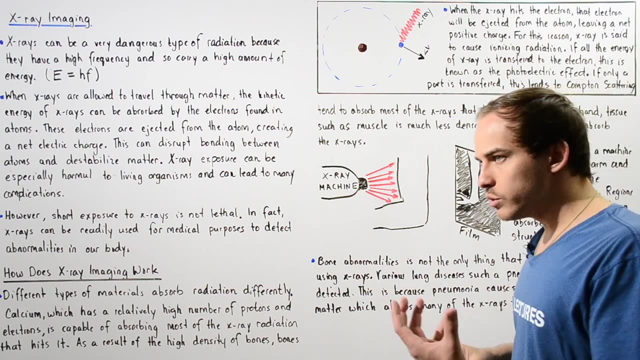 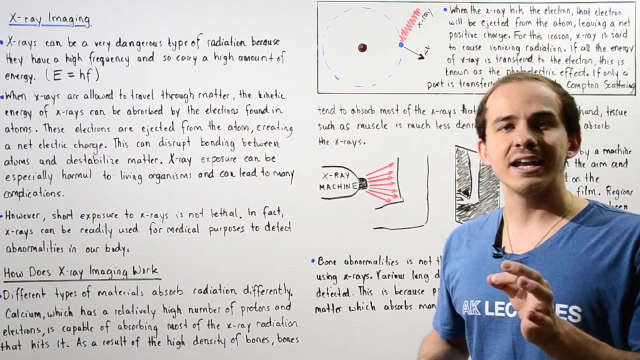 photoelectric effect. If only a part of is transferred, this leads to Compton scattering or the Compton effect, And in both cases this can create many detrimental effects. Now, even though this is true, x-rays do in fact damage the atoms found in our bodies. short exposure to x-rays is not 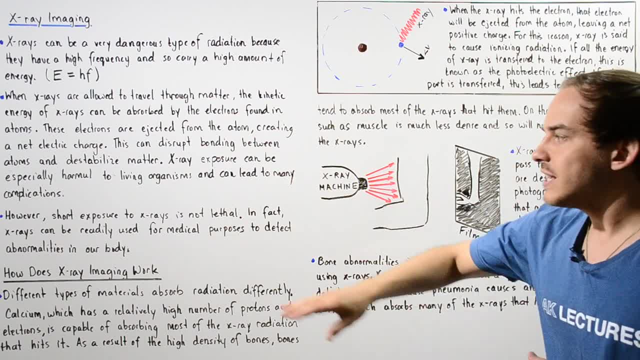 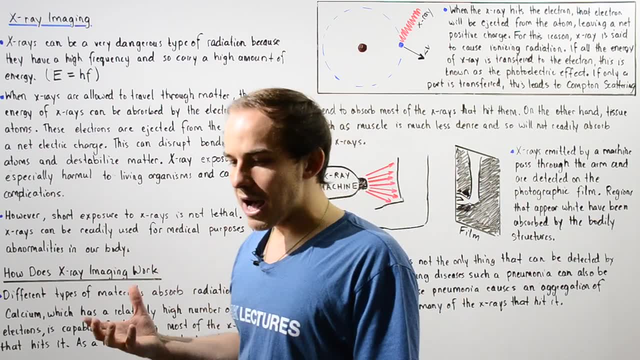 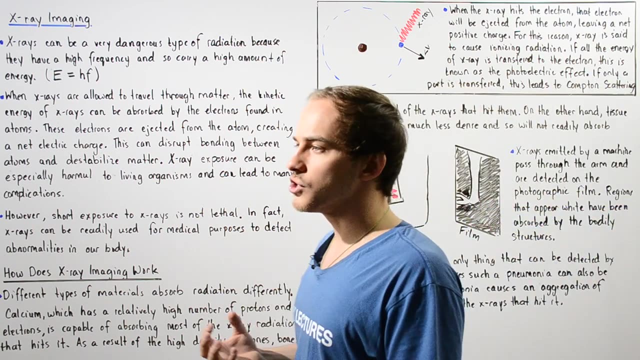 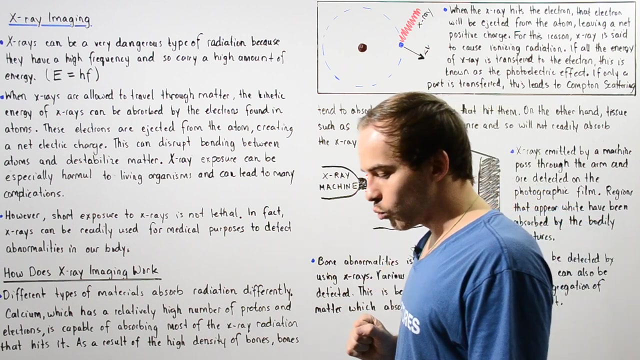 exactly lethal. In fact, x-rays can be readily used for medical purposes to detect abnormalities in our body, and this is called x-ray imaging. So we use x-rays to form images of certain structures found inside our body. Now, how exactly does x-ray imaging actually work? 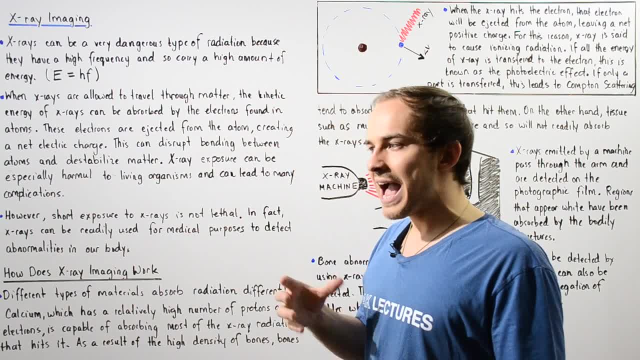 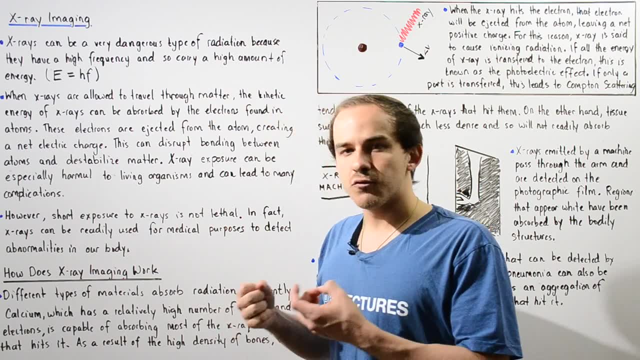 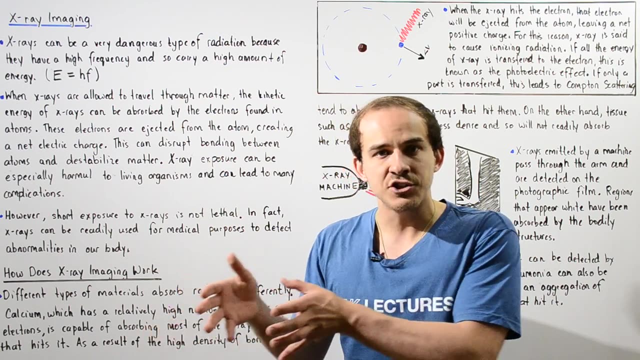 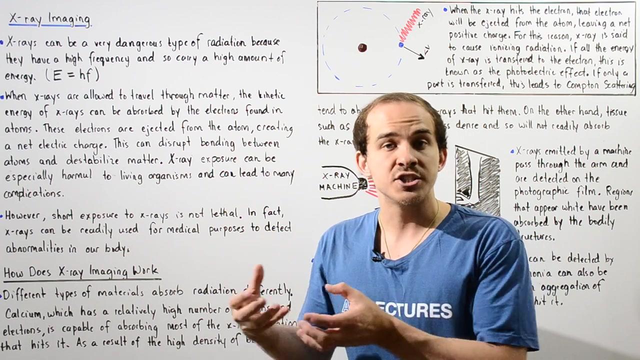 So let's recall some basic information about how our objects actually absorb radiation. So basically, the amount of radiation that any given object absorbs depends not only on the type of radiation hitting that object but also on the atoms that compose it, That object. So certain materials absorb more radiation than others. So different types of 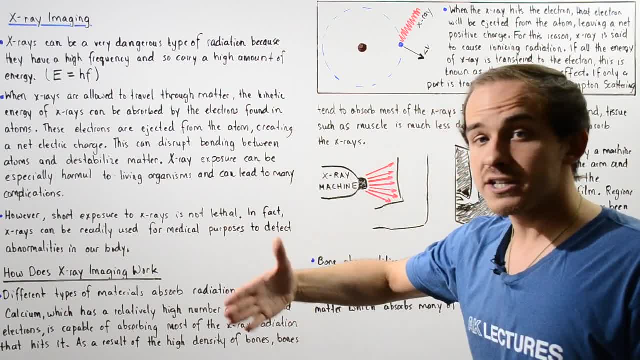 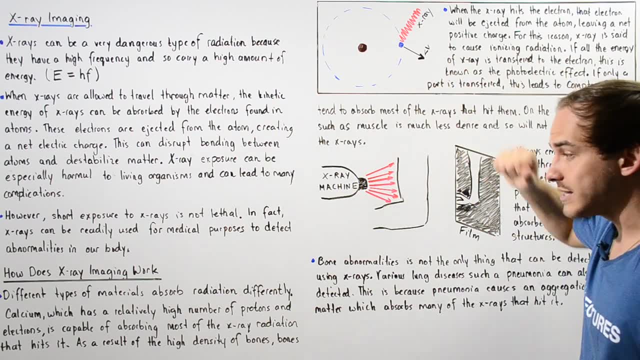 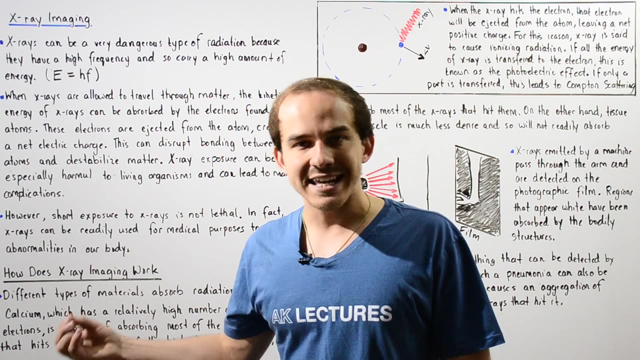 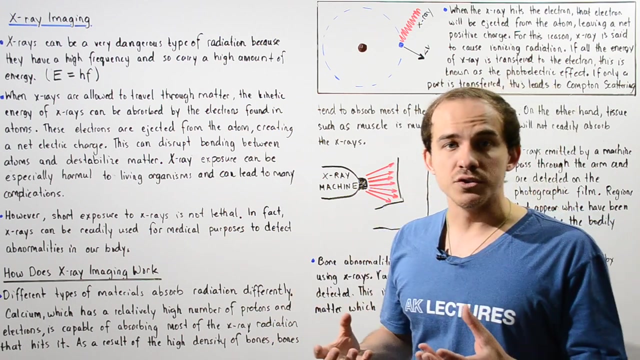 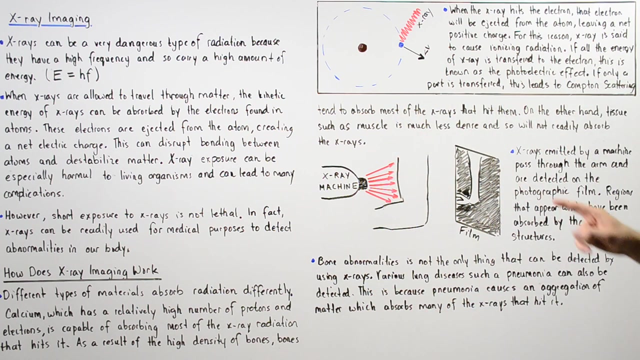 materials absorb radiation differently. For example, calcium, which has a relatively high number of electrons and protons in the nucleus, is capable of absorbing most of the x-ray radiation that is incident on that calcium atom. So as a result, we see, because our bones have a very, very dense concentration of calcium, bones tend to absorb. 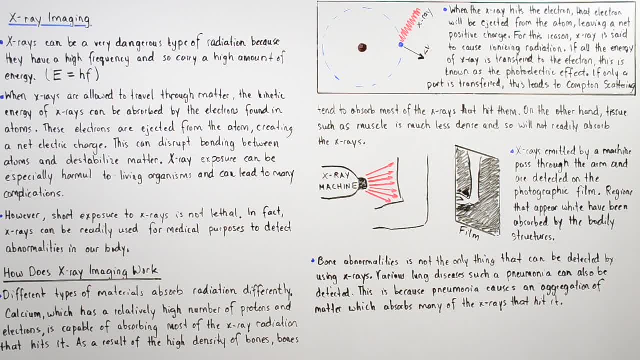 most of the x-rays that hit them. On the other hand, other types of tissues, for example muscle tissue, is much less dense and so will not readily absorb our x-rays. So let's take a look at the following diagram. Let's suppose we have the following arm: 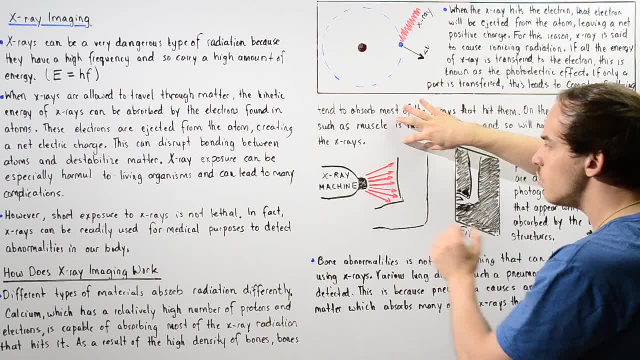 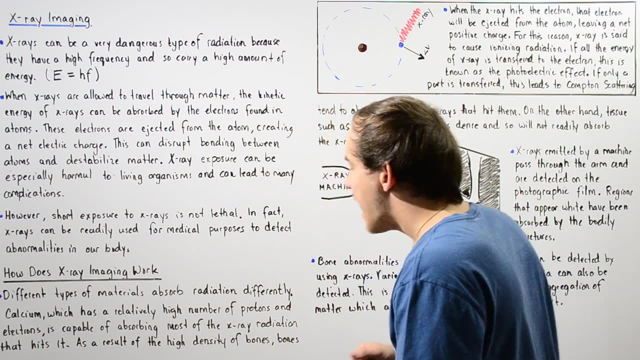 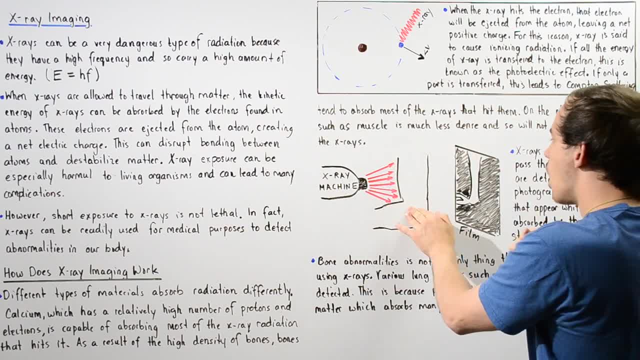 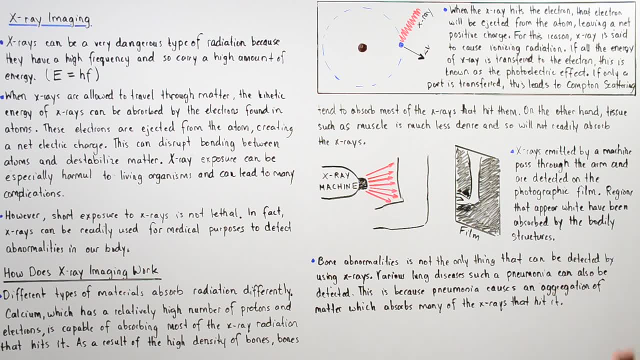 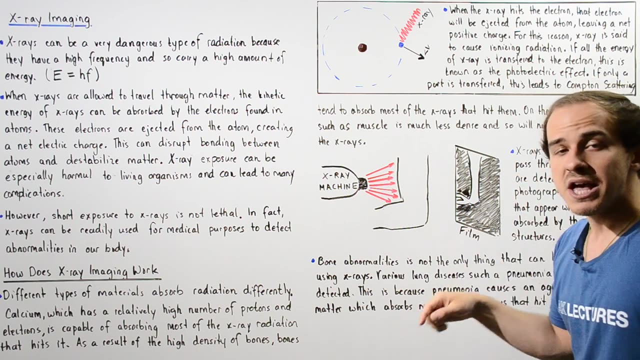 as shown, and travel through this person's arm. Now, in back of the person's arm, we have some type of film, some type of photographic or fluorescent film. Now, basically, when the x-rays- if the x-rays actually hit the film, they will react with the film and basically cause dark regions. However, 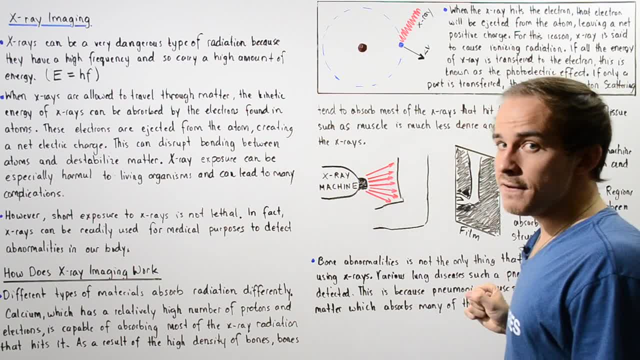 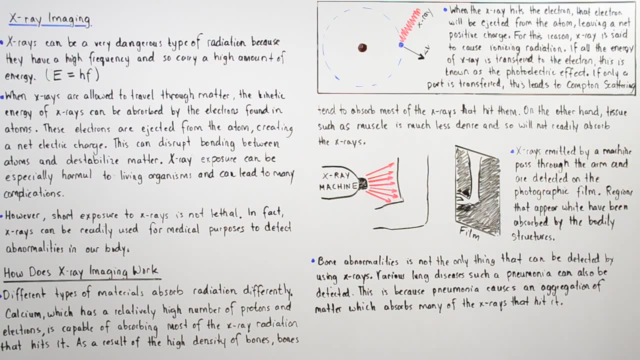 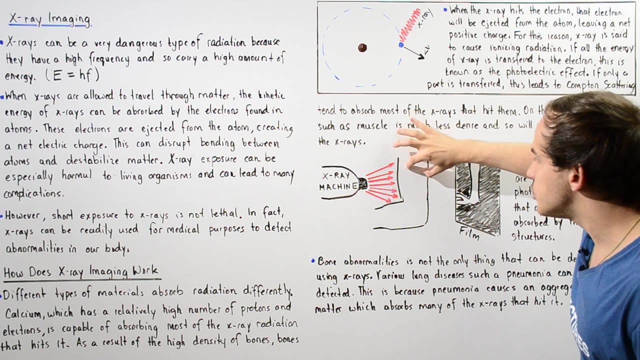 if the x-rays do not actually reach our film, this film will remain white. So we see that x-rays emitted by the machine pass through the arm and are detected by the photographic film. However, the regions of our body that absorb most of that x-ray, most of that radiation, 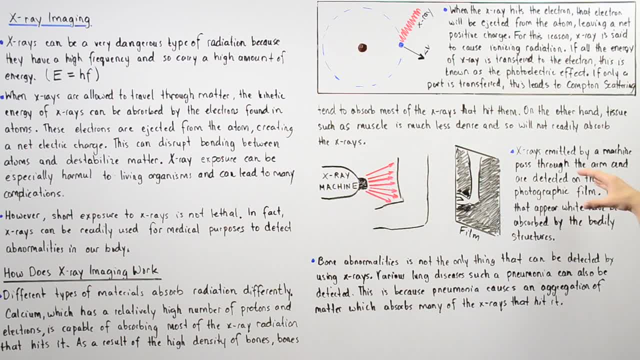 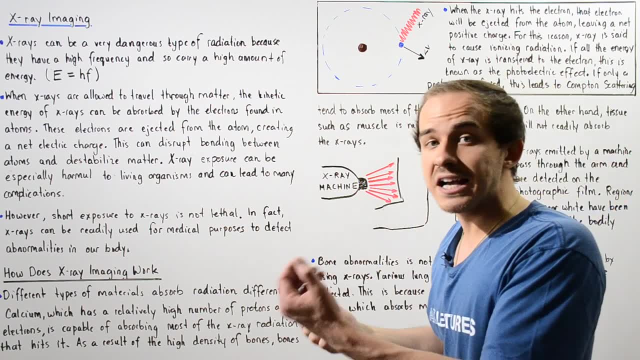 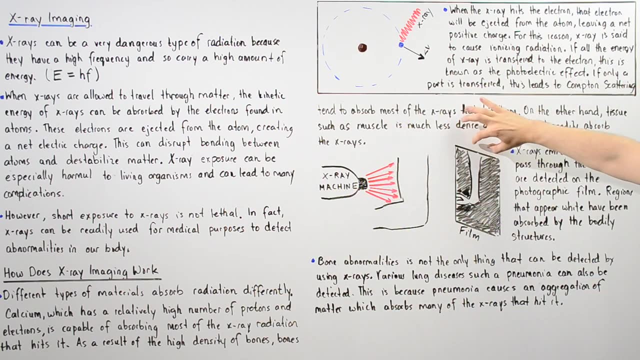 those x-rays do not actually end up passing through and do not end up on the film, And that's why, for example, bones that do in fact absorb most of that radiation as a result of the high density of calcium, end up appearing white on our screen, on our film. So 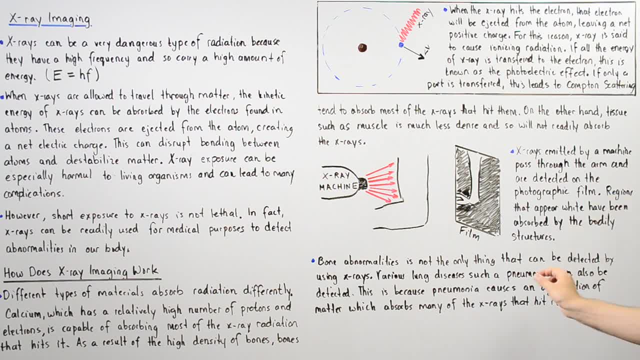 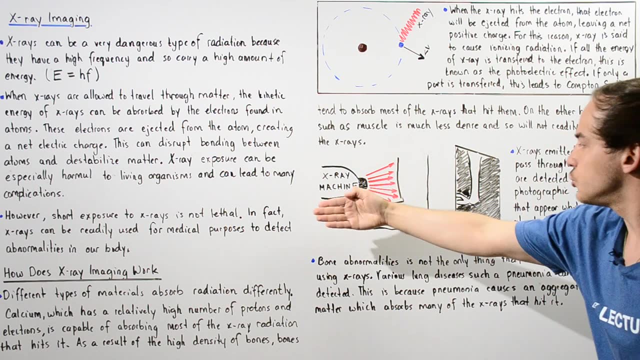 regions that appear white have been absorbed by the bodily structure, So the x-rays have been absorbed and the x-rays do not actually end up falling on our film. But these dark regions represent the regions in which x-rays do actually pass through the body and are therefore not 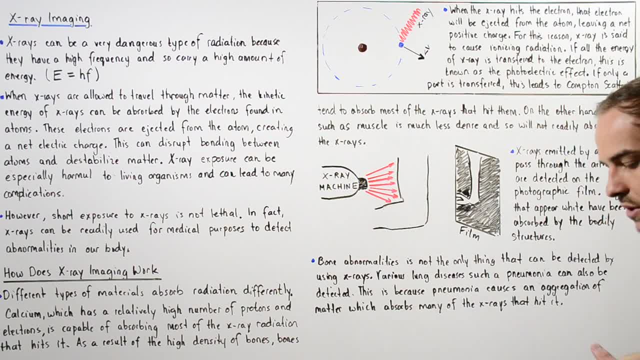 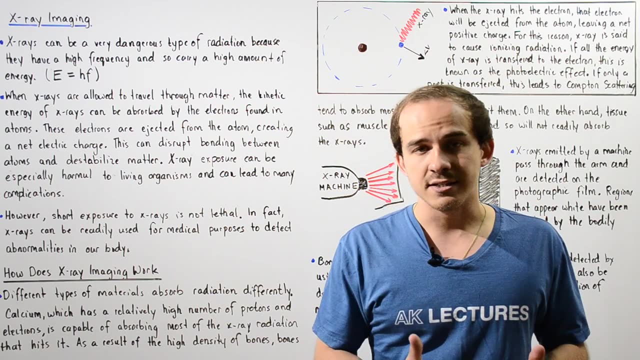 absorbed and are able to get onto our film. So we see that bone abnormalities, for example bone fractures, is not the only thing that can be detected by using x-rays. Other things, for example lung diseases such as lung cancer or pneumonia, can also be detected. This is because 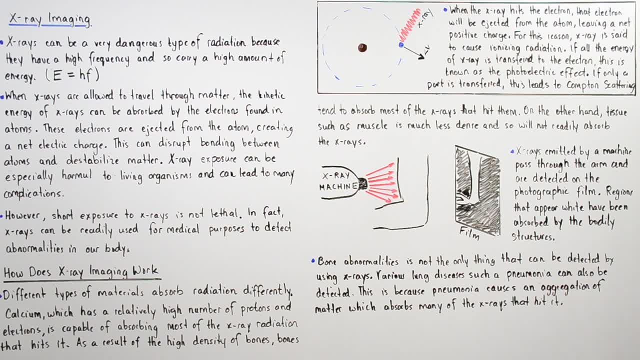 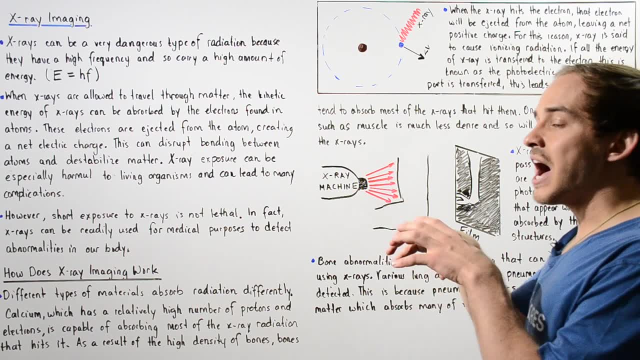 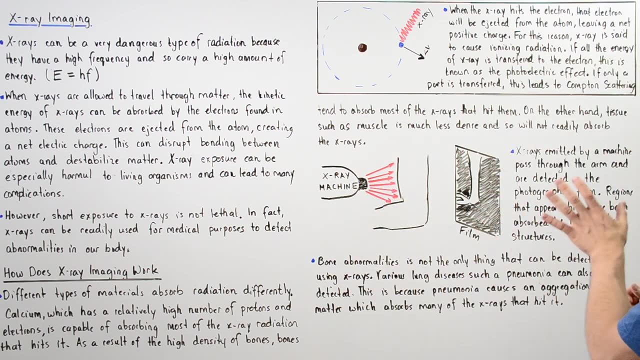 in the case of pneumonia. pneumonia causes an aggregation of matter inside our lungs And this aggregation of matter, this high concentration of matter, readily absorbs the x-rays. So, for example, bone fractures is not the only thing that can be detected by using x-rays, or vs and so on, And this reasons is that a large portion of what we see 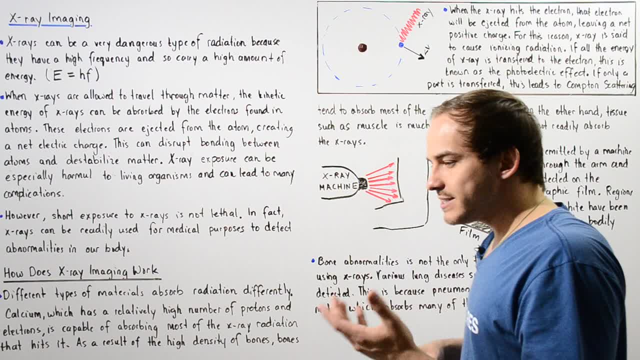 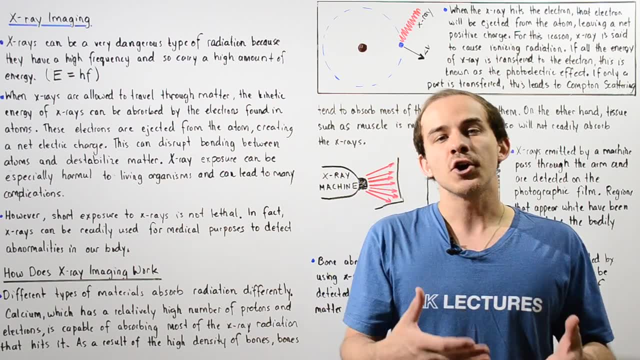 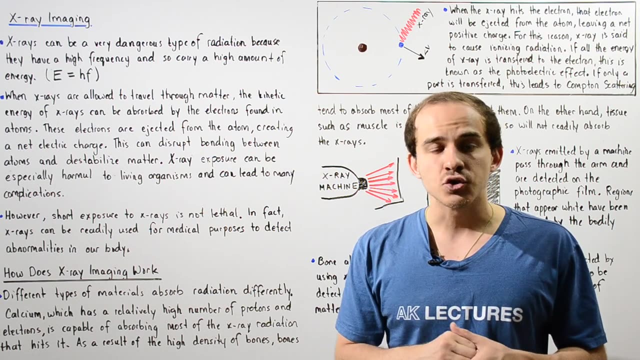 is the cause of Ramadan, the football. We also see a normal examination with tutoring from Professor Twice films and doctors who can tell us where did they get the x-rays? To do more testing? take a look: this x-ray of our lungs and the other x-rays on both of our lungs are the first imagesethat we can período. 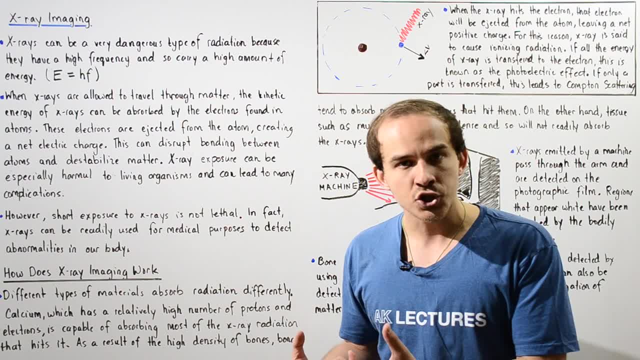 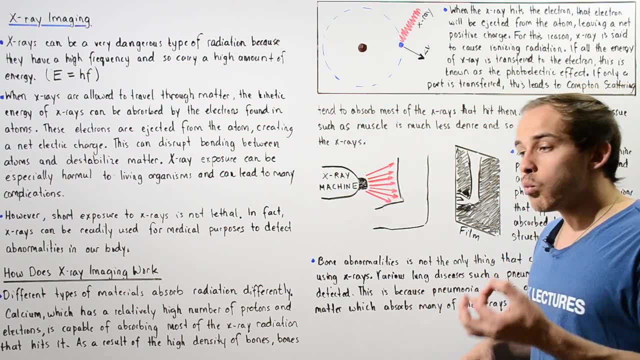 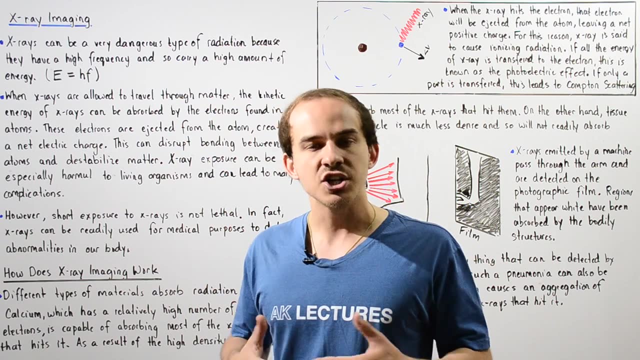 do if you see anything on our X-rays. so at least three times of the x-rays So we notice that. So if your lungs are in fact punctured, they will collapse, and so that means fluid can get into your lungs and when you take the x-rays that fluid can basically appear on our x-ray as white regions. 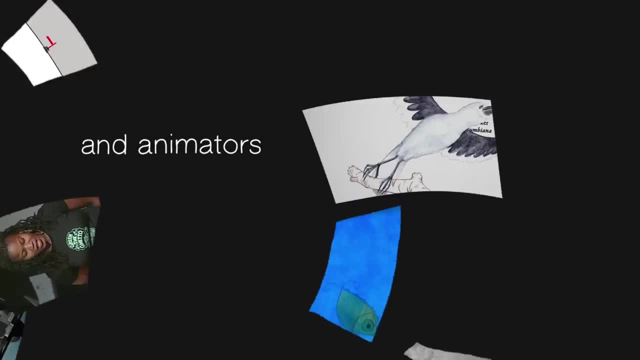 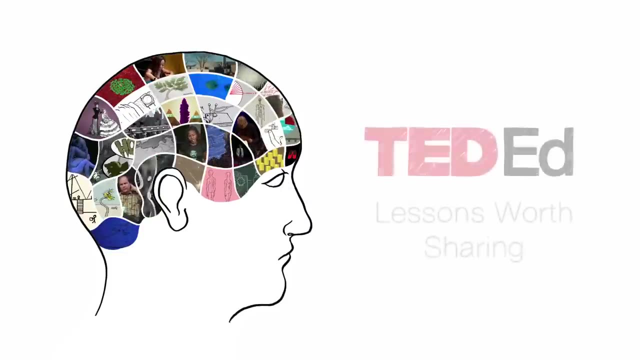 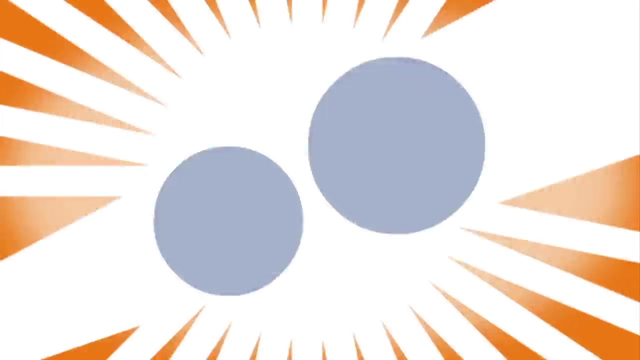 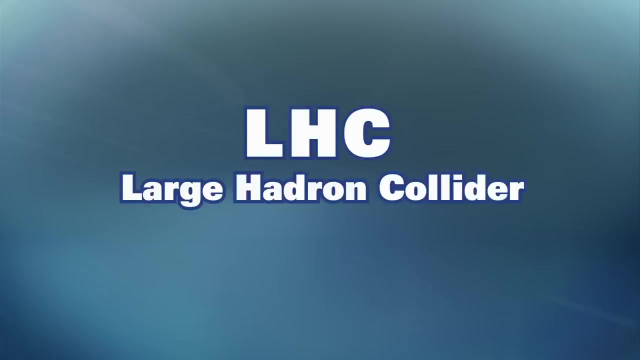 One of the grandest scientific tools ever made by mankind is called an atom smasher, And I mean literally grand, The biggest one ever built. the Large Hadron Collider, or LHC, is a ring with a circumference of about 18 miles, That's more than the entire length of Manhattan. 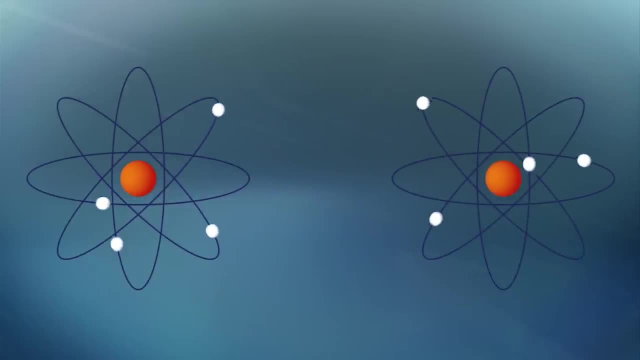 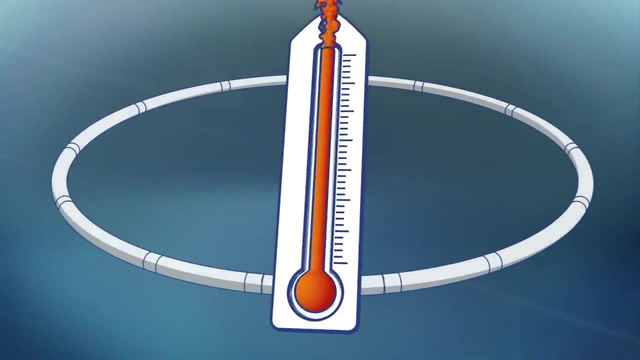 So what is an atom smasher? It is a device that collides atomic nuclei together at extremely high energy. The most powerful one scientists have ever built can heat matter to the hottest temperatures ever achieved, temperatures last seen a trillionth of a second after the universe.